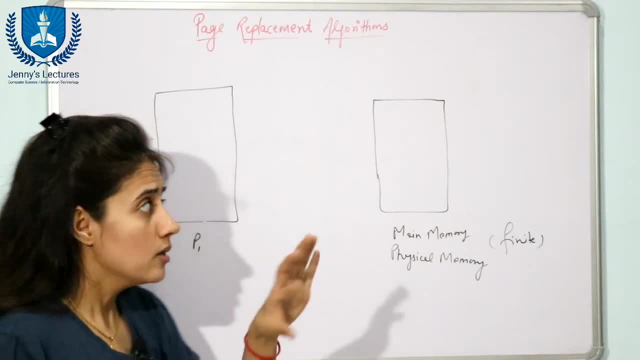 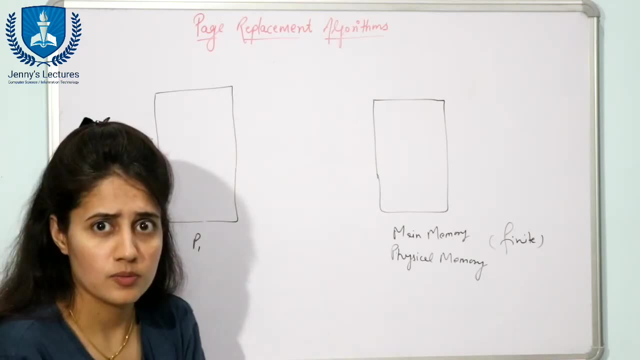 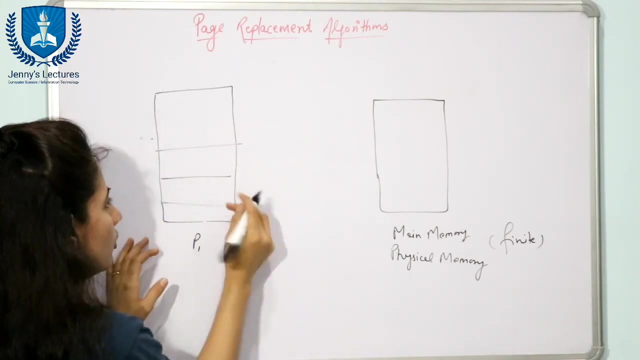 can? we can load only some part of the process. see, because when cpu is working, cpu, cpu is executing this process. it is not like that cpu is executing the complete process. maybe cpu is executing only this part of the process. maybe cpu is executing only this part of the process. so it is. 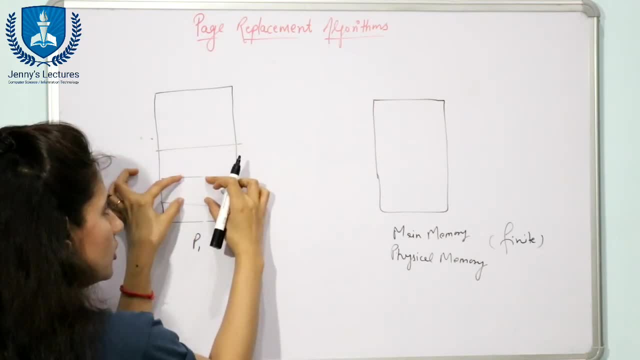 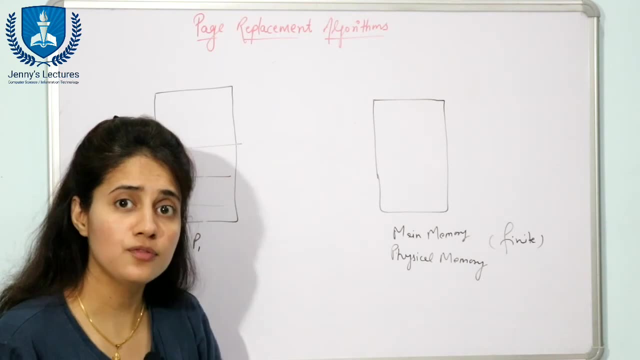 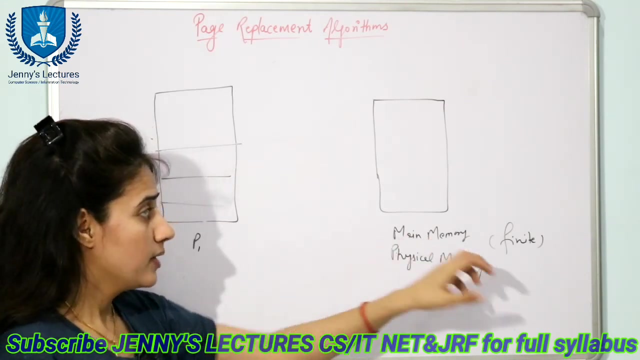 better to is: it is better to load only this part or this part to main memory rather than loading the entire process into the main memory. if you can implement this funda for memory management, then what? what is the benefit of this thing? because, as the size of this memory is finite. so if you 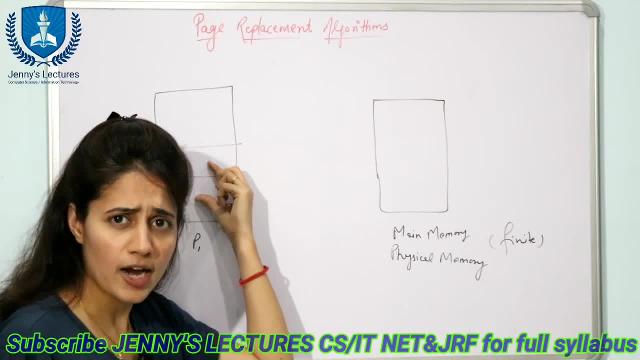 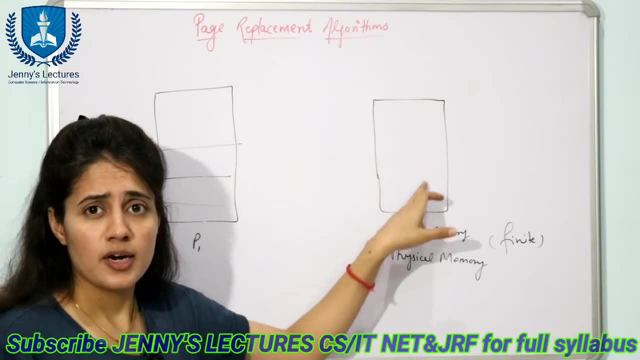 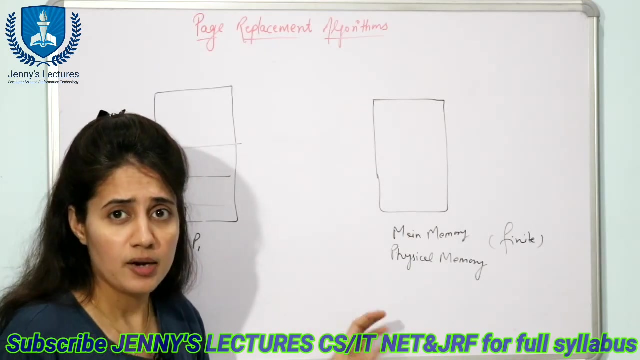 implement this funda, only the required version of the that process is to be loaded into the main memory. then what will happen? many, many processes can reside in the main memory at same time, because if you load the complete process, then it will take larger space in the main memory and maybe at one time maybe two processes can be there. 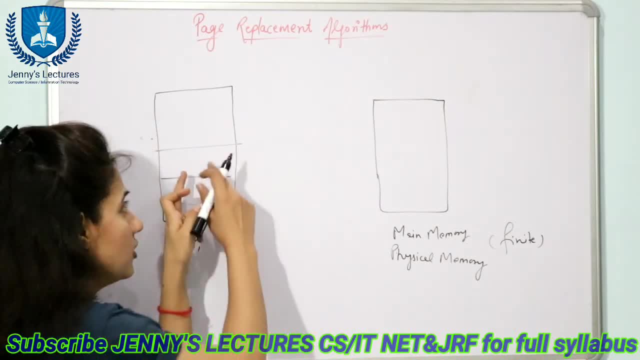 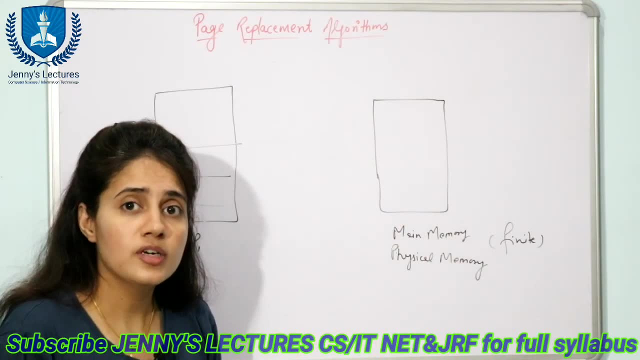 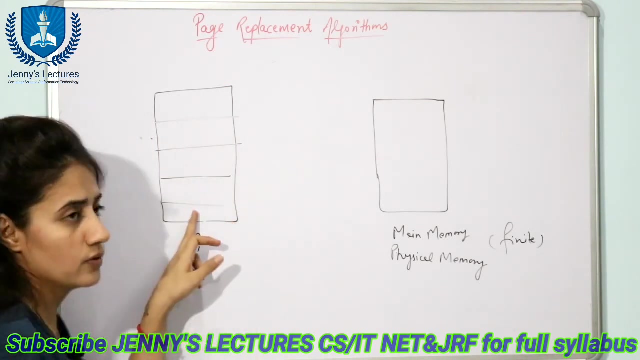 in main memory. three processes can be there in main memory and if you apply this funda, then maybe at same time five, ten, fifteen processes can reside in main memory. okay, now how this funda is to be implemented. simple trick is, if we divide this process into these portions, equal sized portions. 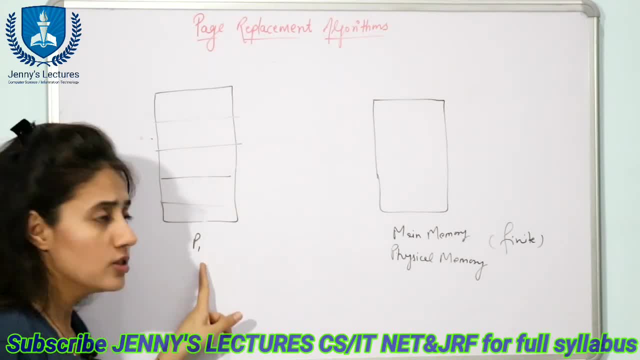 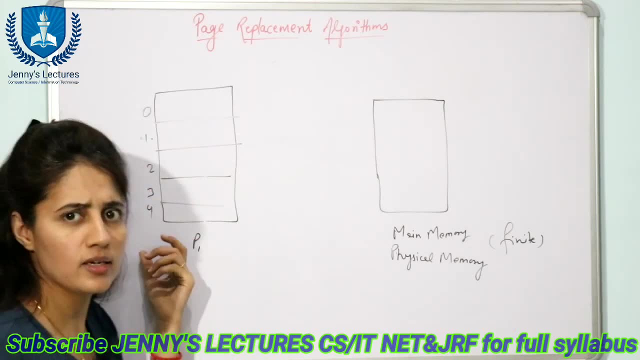 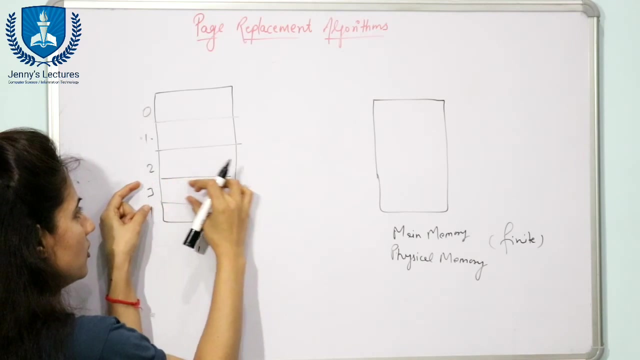 and this. this is known as pages. so process is divided into equal sized pages. this is suppose page zero, one, two, three, four we are. we are taking page number at some time. cpu is executing this process and cpu needs only the page number three. so only this page is to be loaded. 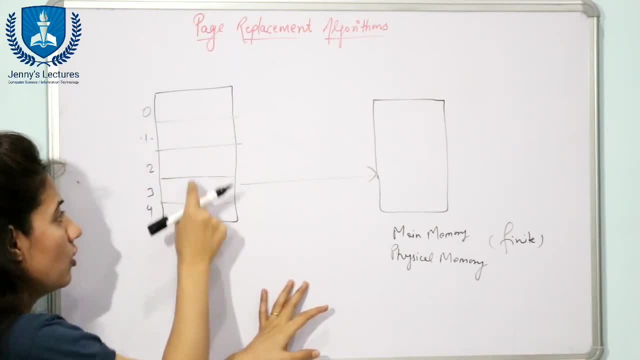 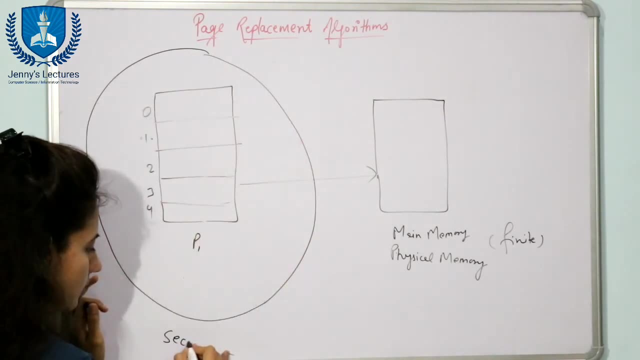 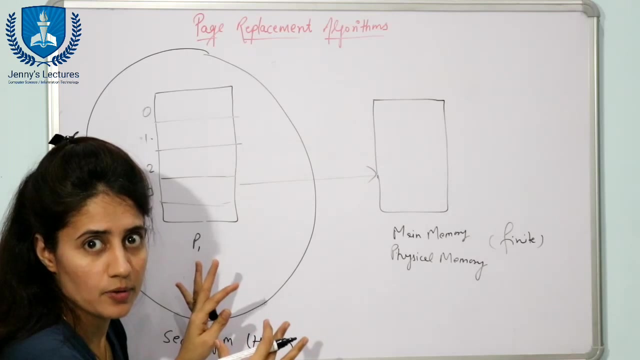 into main memory. these pages will not be loaded into main map, so these pages will will be in secondary memory, like that. suppose this is our secondary memory, or you can say hard disk. okay, somewhere in secondary memory, all the pages of this processes. they are in secondary memory and 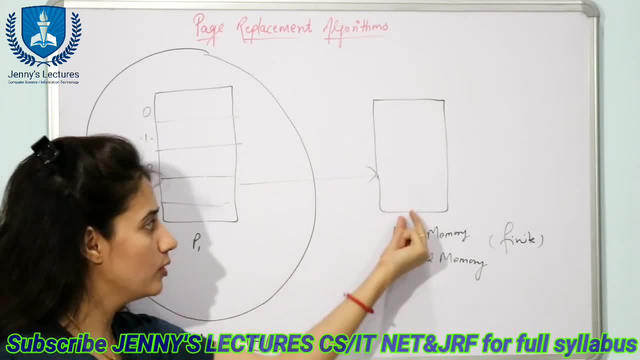 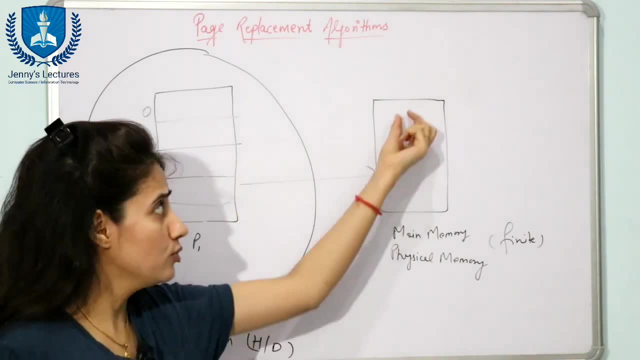 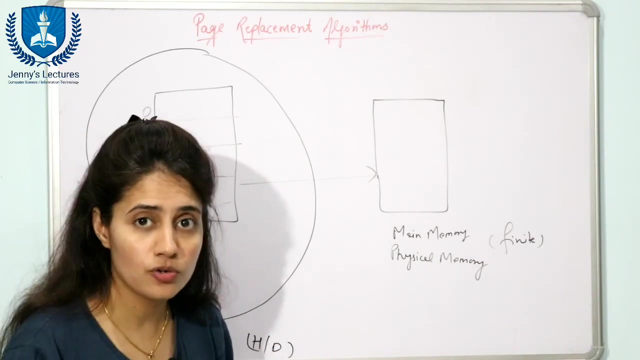 when the cpu needs a particular page, then that page is to be loaded into main memory. this kind of funda is also known as demand paging, and when you apply this funda then many processes can be there in main memory. so it seems that that main size of main memory is very large, but actually that's not true and that thing is. known as what? virtual memory, because that is virtually. it seems that the size of main memory is very large because many processes can be there in main memory. why so? because we are not loading the complete process into the main memory, we are just loading the required pages into the. 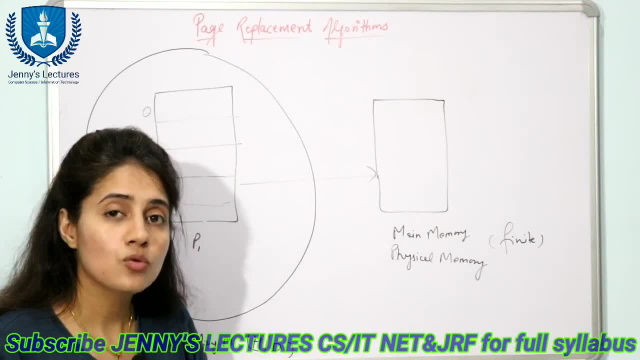 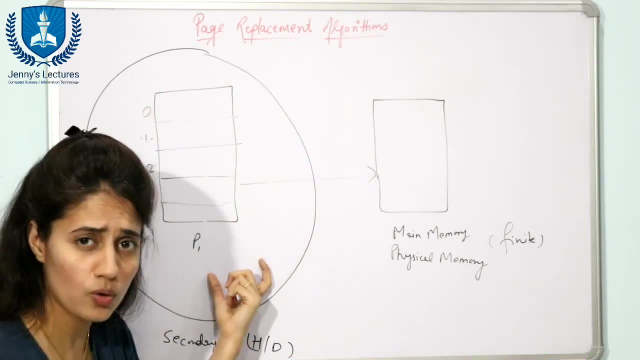 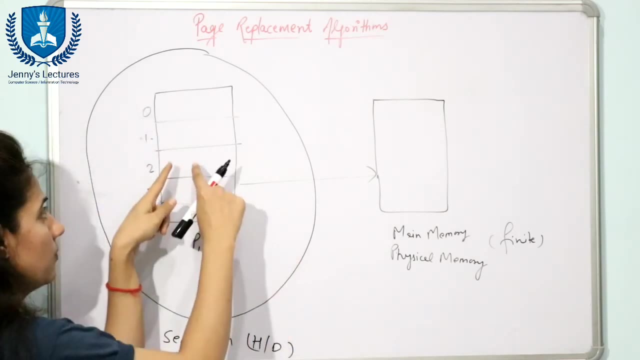 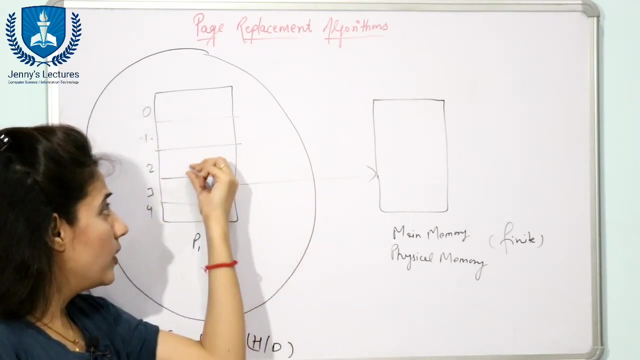 main memory. okay, so that that thing is known as virtual memory. actually, virtual memory is: see this, this, some portion of hard disk is known as virtual memory. now, see if at some point of time cpu needs this page number two of this process, p1. now, if this requested page is available in the main. 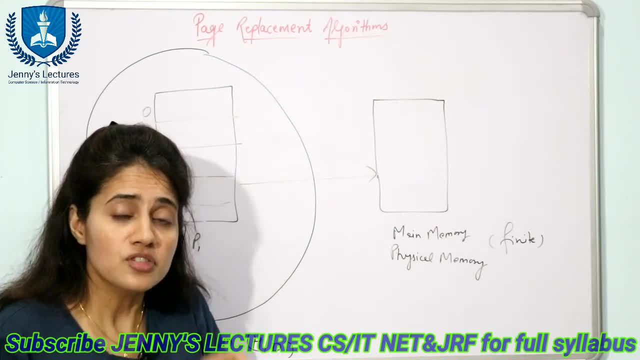 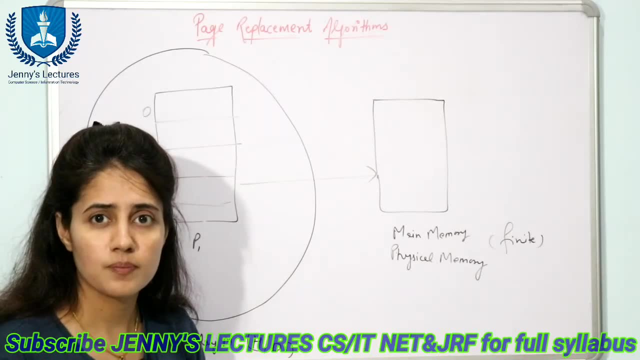 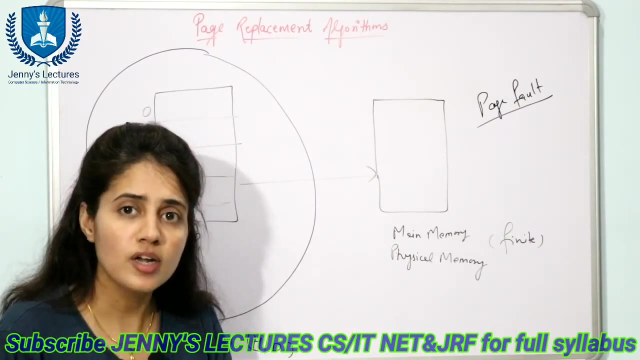 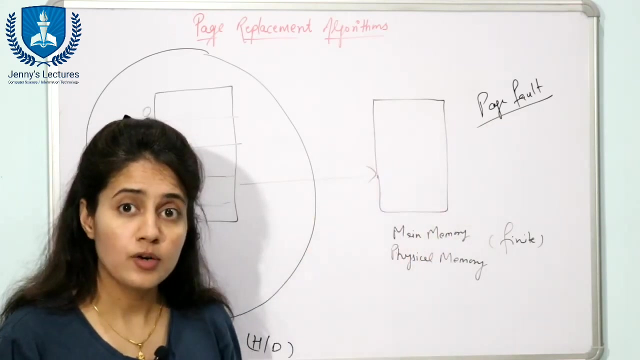 memory, then normal execution will be there. if some, if suppose this page number two is not load, not there in the main memory, then that thing is known as page fold. if the needed page is not available in the main memory, then that thing is known as page fold. now, if page fault occurs, then what will happen if operating system finds that? 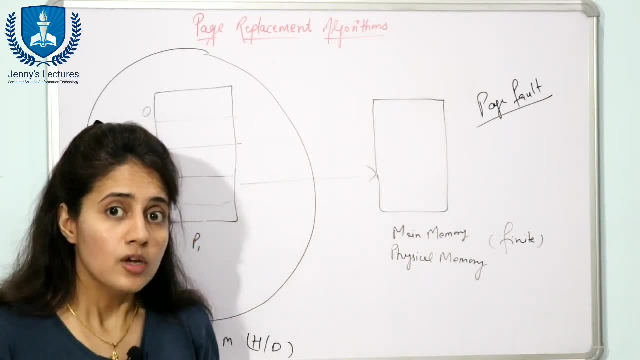 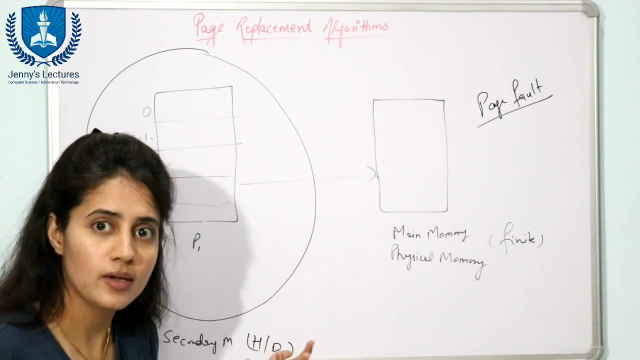 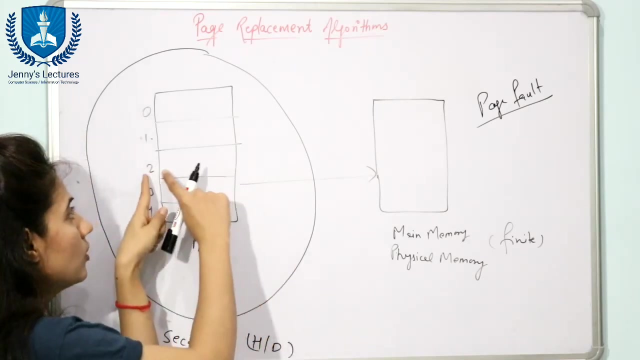 that particular page is not in main memory, then what operating system will do? first of all, operating system will detect with hard disk, where the process reside in hard disk, it will find, okay, and it will find that page of that process, the needed page of that process, and it will load that page into main. 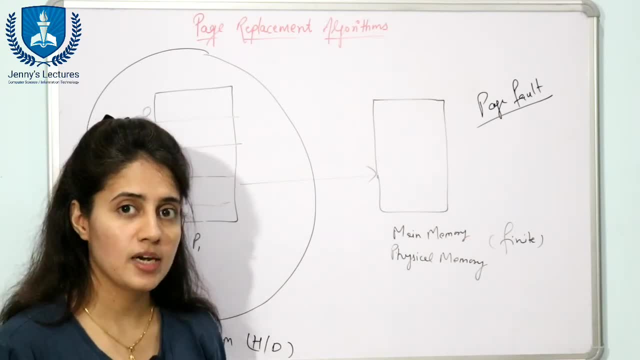 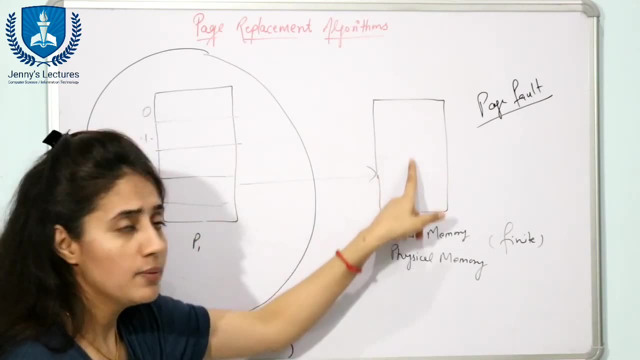 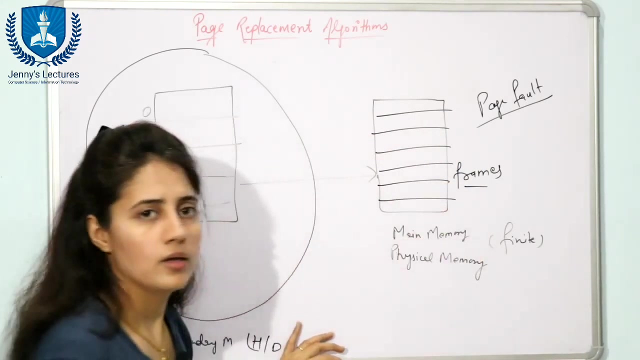 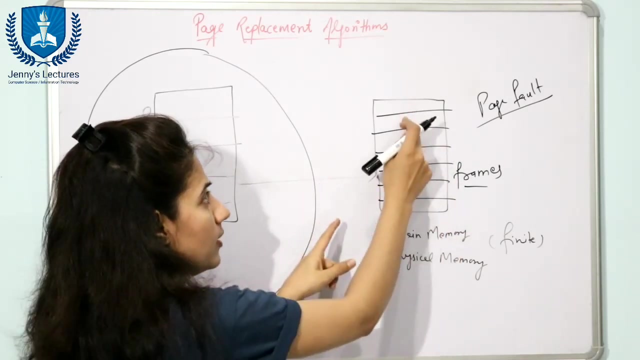 memory. now, if the situation is something like that, the main memory is full, see, the process is divided into equal sized pages and the main memories is divided into frames like this: equal sized frames. if the memory, if this main memory, is full, all the frames are having some pages. so if this main memory is full, then you cannot put the requested page, the page number two, in this main memory. then what operating system will do? obviously some page has to be swapped out into secondary memory so that the new requested page can be swapped it into main memory. you see page. 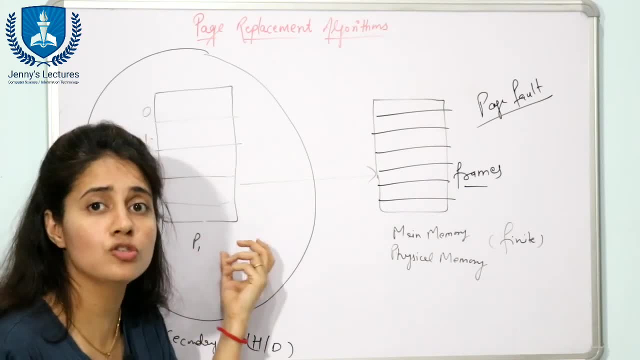 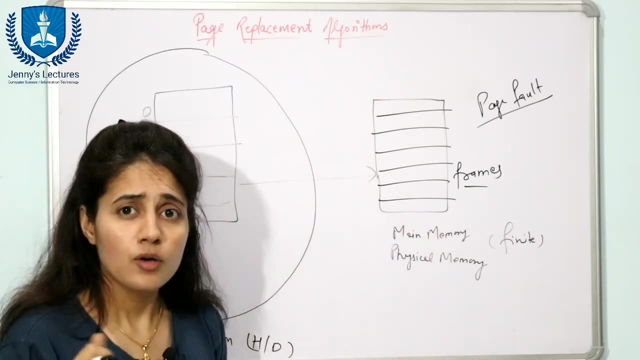 you have to pick it up from here and put it into secondary memory from main memory. that is known as swap out. okay, and when you put a page from secondary memory to main memory, that is known as swapping. now the question is which page is to be replaced. the operating system will choose which. 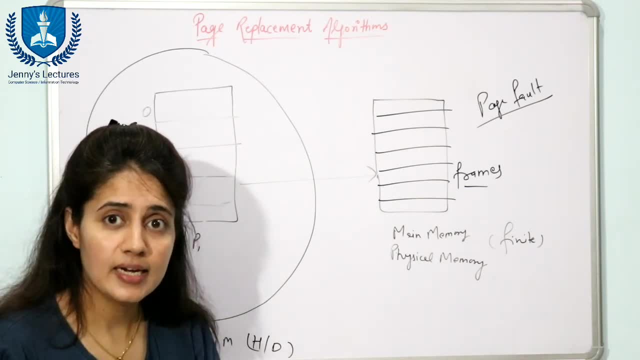 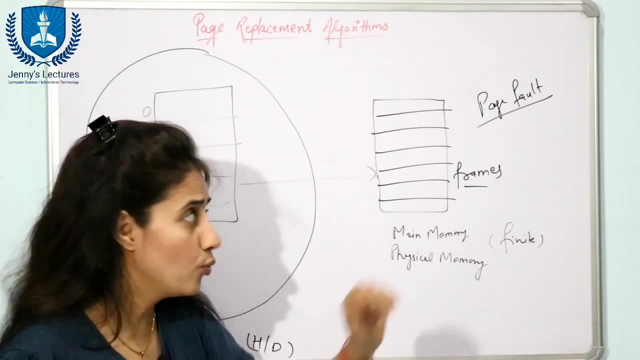 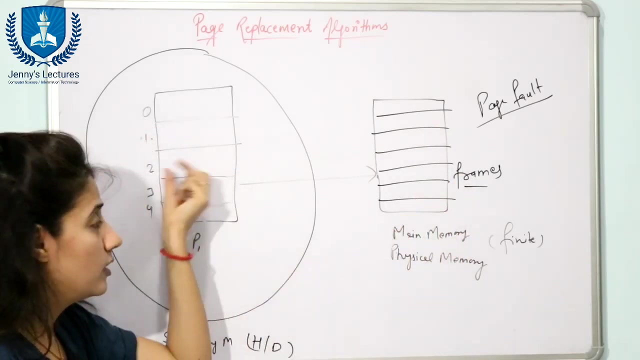 page to swap out. that thing is decided by page replacement algorithm. so there are many algorithms to decide which to decide this thing, that which page is to. if main memory is full, all the frames are full, then which page is to be replaced with this new page? for deciding this thing we have 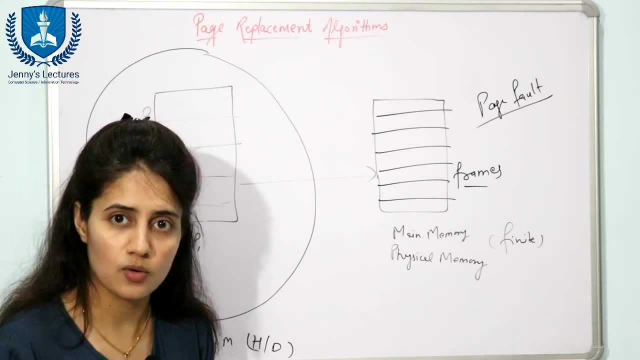 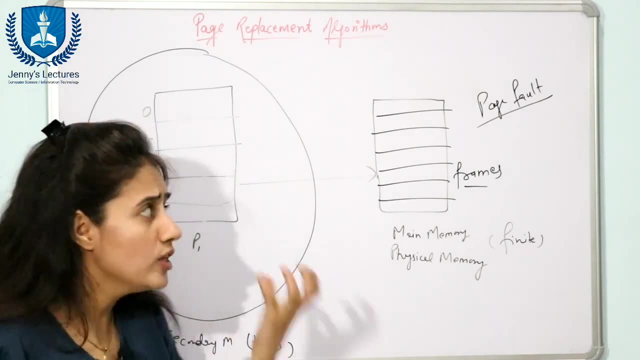 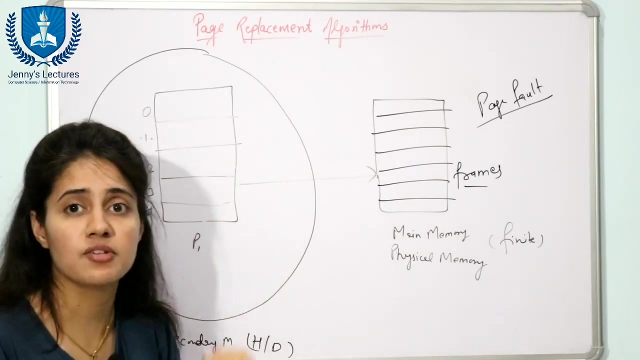 many types of algorithm. so in this video we will discuss first in, first out algorithm. now one more important thing is how operating system knows which page of which process is in main memory and which page of that process is in secondary memory. obviously the operating system has to keep this. 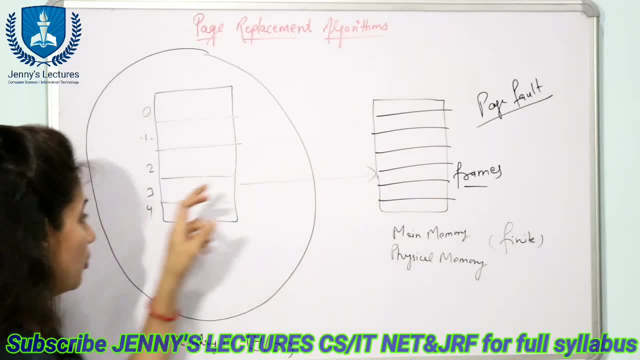 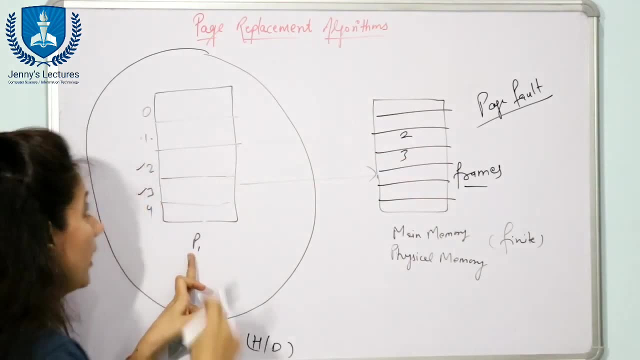 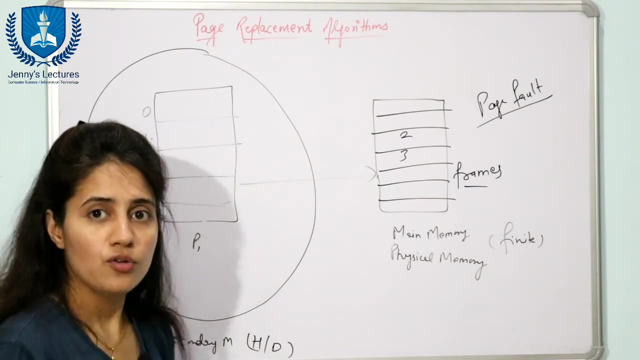 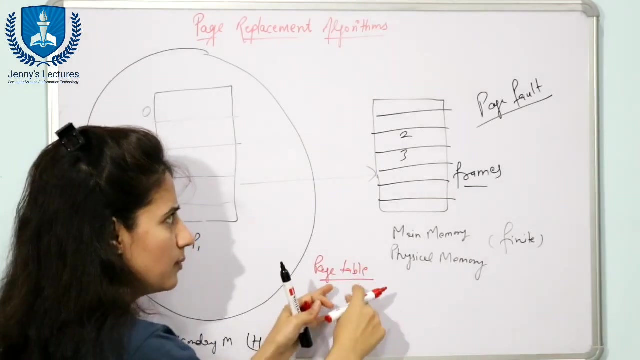 information also, that which page is, in suppose the page of p, this process, p2, this two or three pages are in main memory and this 0, 1, 4 are in secondary memory. okay, so operating system keeps this information also and for keeping this information one page table is there, so this page table is also. 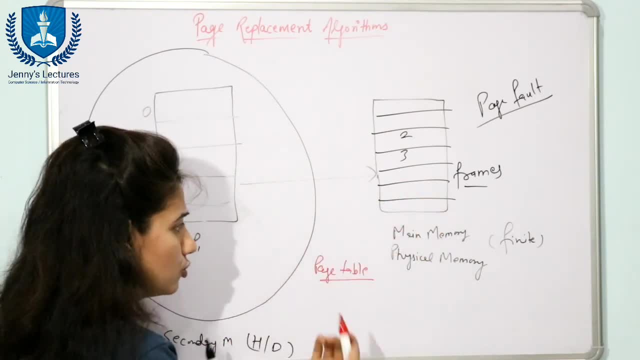 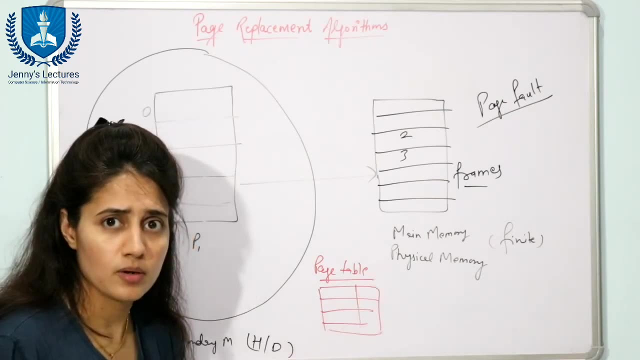 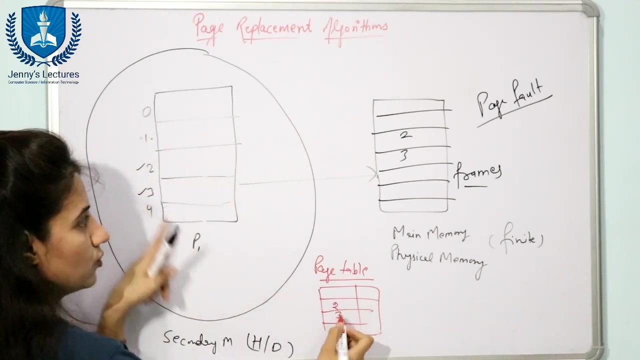 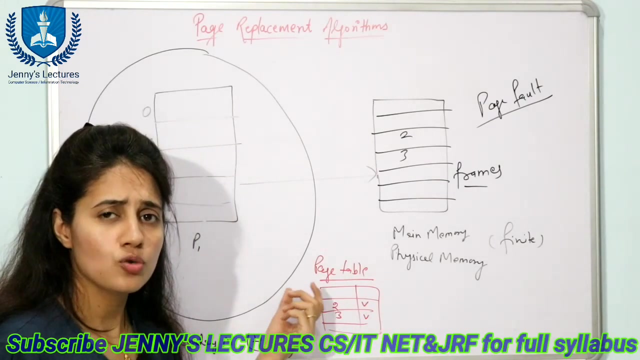 reside in this main memory- okay, somewhere. so maybe so many information are stored here. so this page is not steroid. this page table is there. however, if we repair- and here this is space table- many, many information are stored in the space table. i am just telling about valid and invalid bits. if this page number 2 and page number 3 is in main, 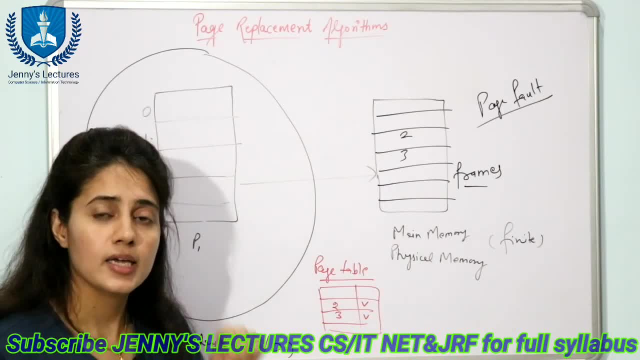 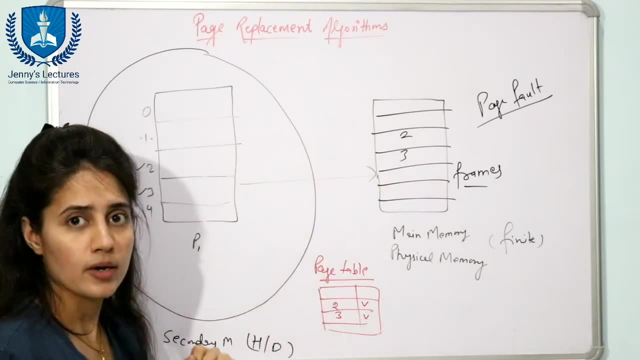 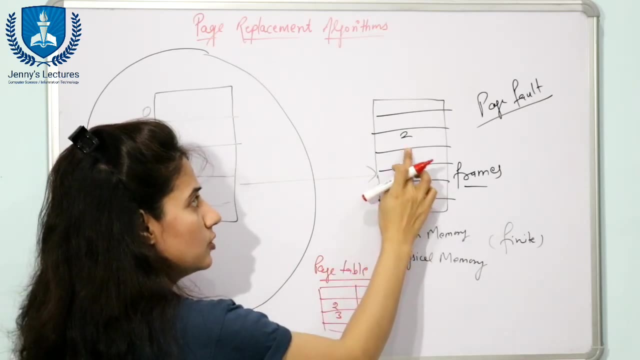 memory, then we set this bit to valid and if if particular page is not there in this memory, then main memory is completely full and you have to swap out some page from here to here and operating system, using some page replacement algorithm, operating system chose this three page number. 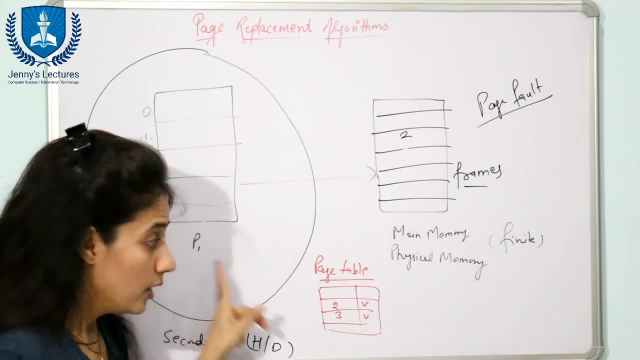 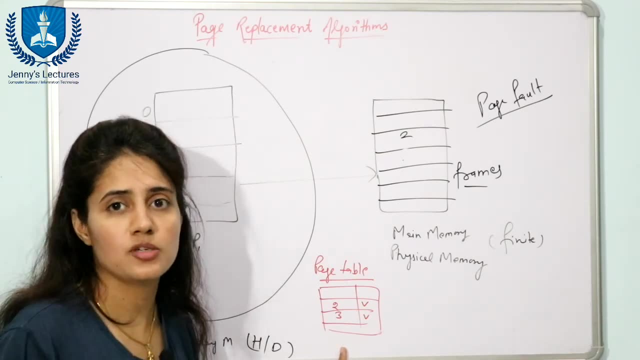 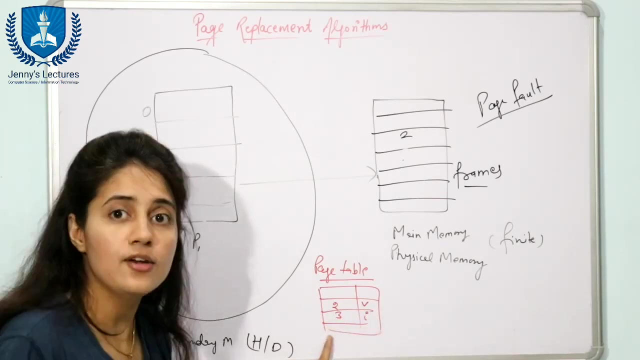 three to swap out in secondary memory. now the operating system will also update this space table it have. it has to update the space table. okay, so the bit corresponding to this page, number three, is set to invalid. now, why invalid? because this page is not available in main memory, right? 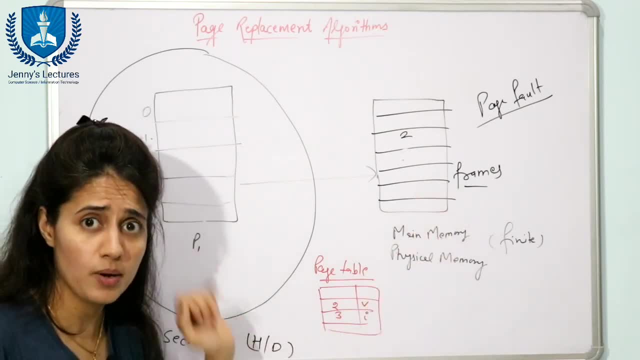 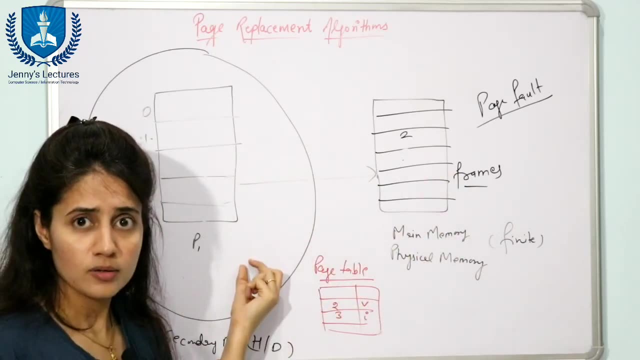 now because this space has been swept out to secondary memory. so this is the processor. when a page fault occurs, then operating system will do. operating system will first of all contact to the hardware to locate where that process is, where the page is. second thing is then operating system will. 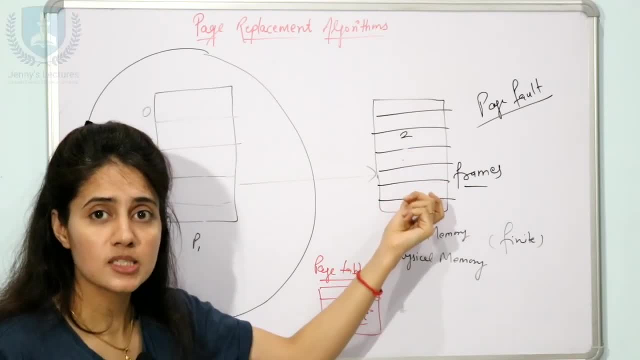 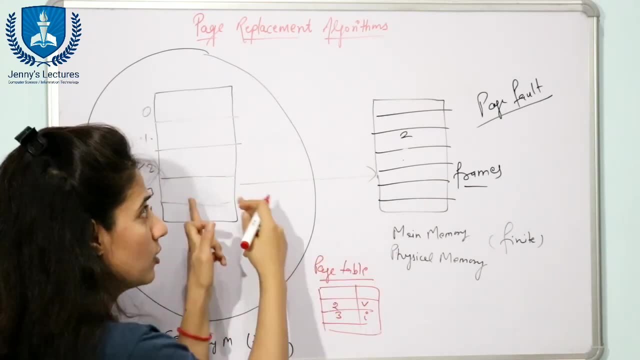 choose the victim page, which page is to be replaced, or you can see which page is to be swapped out to secondary memory. then that page can be replaced when operating system swap out to secondary memory, page would be swapped out from that secondary memory and the new requested page would be. swapped into the main memory plus operating system will also update this page table. the corresponding bit to that page which has been swapped out is set to invalid. okay, and the corresponding bit to the page which has been swapped in is set to valid. so this is the processor. so, before going to that algorithm, i just want to tell you one more thing, one. 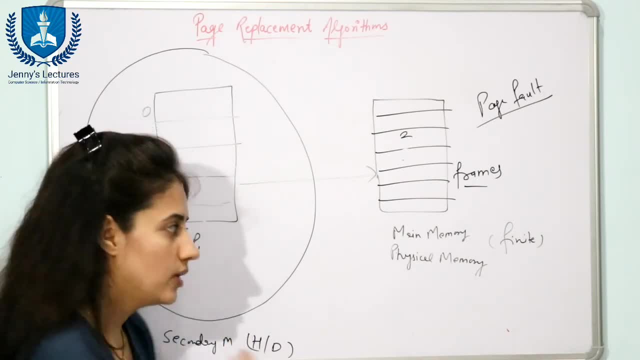 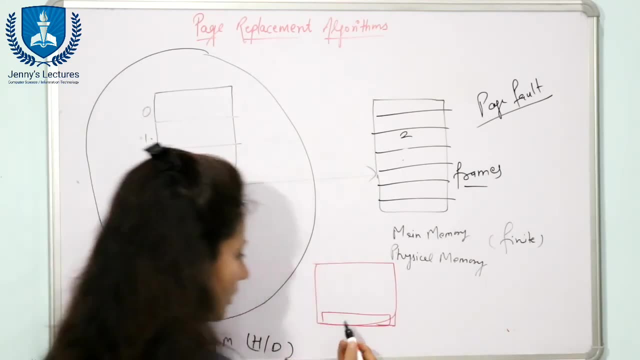 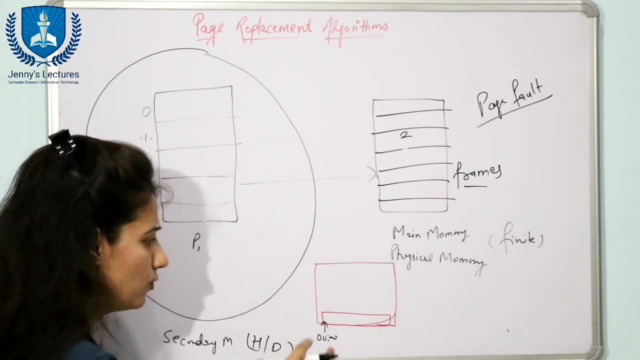 example of that page fault. see, when you open some movie in vlc player, suppose this is your vlc player or this one is your screen. so here you have some that bar and the cursor is now at this place at time 00 and movies. you have started the movie. now suddenly, if 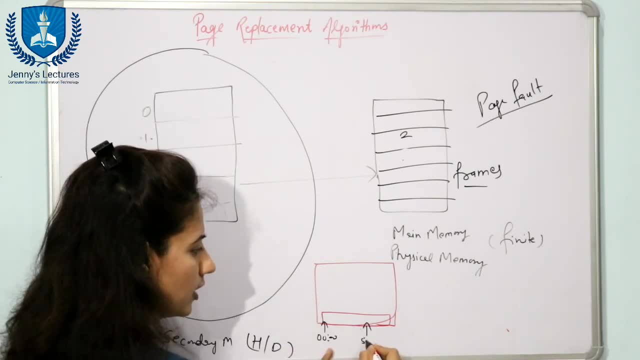 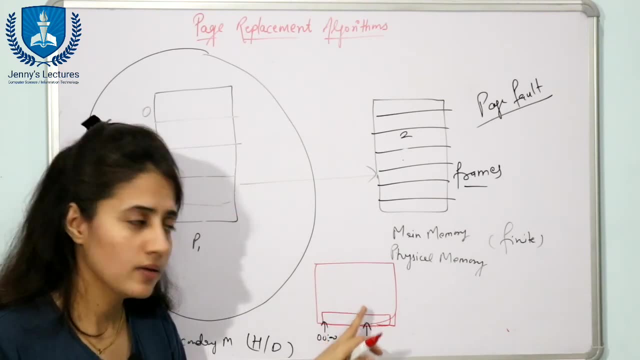 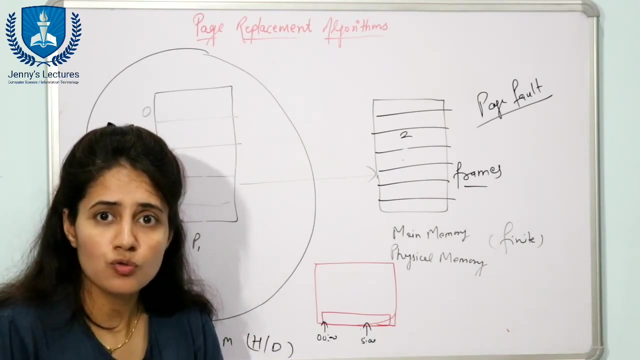 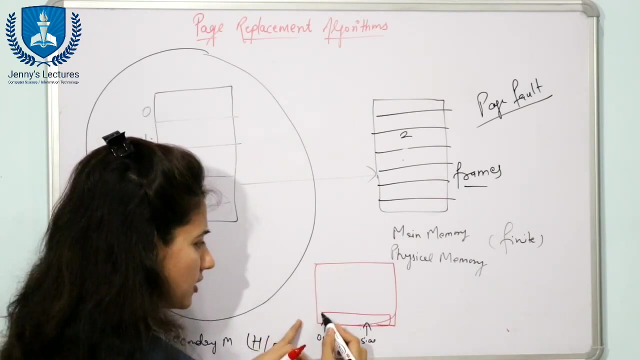 you forward this cursor here to here, maybe suppose at 5 minute, then i guess you have noticed that that vlc player will not play this movie instantly. okay, it it takes some time. it takes maybe one second, two, second or three seconds. why so? because that is page fault. you can say: you can take something like this: this complete 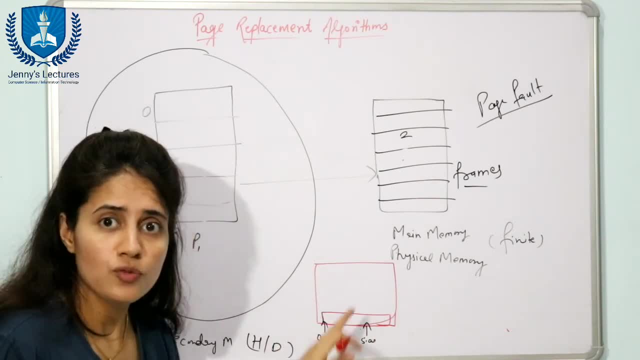 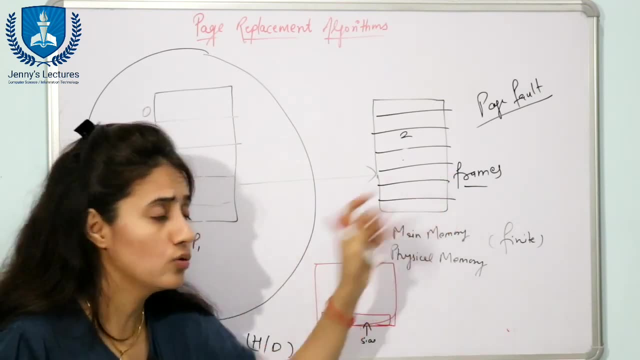 is known as a process, so this complete entire process will not be loaded into main memory when you start the movie. okay, all the pages of that process will not be loaded into main memory when, when- the operating system is using paging technique for memory management. in that case only. 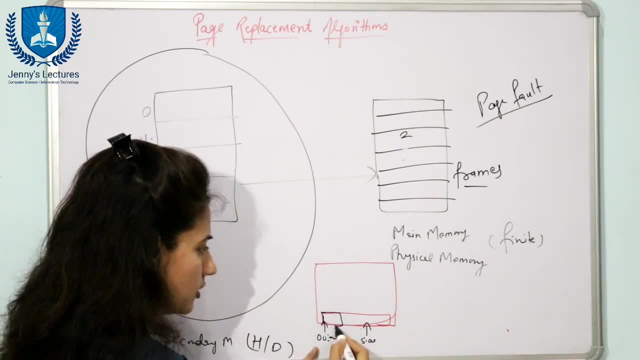 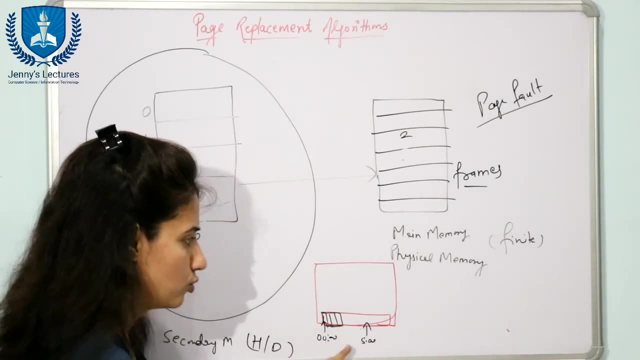 so maybe at some point you will notice that this process will not be loaded into the main memory. when you get starting, the operating system will load only some pages like this, maybe from here to here, okay, and you suddenly put the cursor to here, so this page is not. 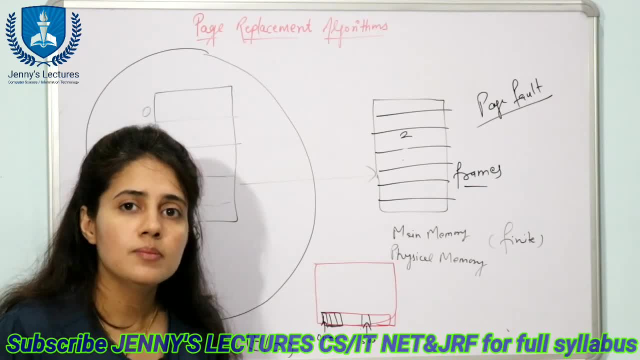 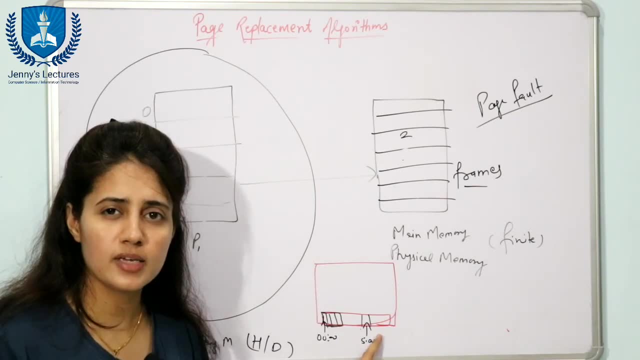 there in the main memory. so that is why it takes some time to load this page. maybe time for swap in and swap out. that is why it takes vlc player takes some time to play the movie from here. so see, so for page replacement, there are many algorithms. now which algorithm is? 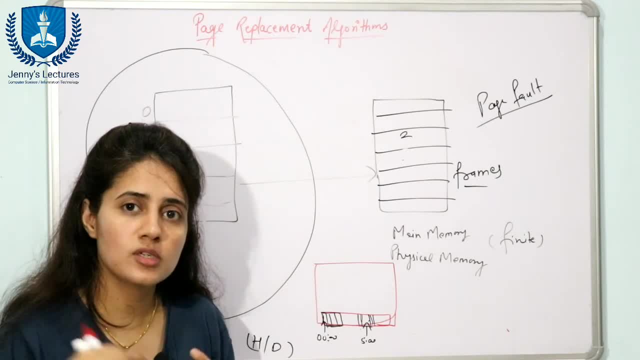 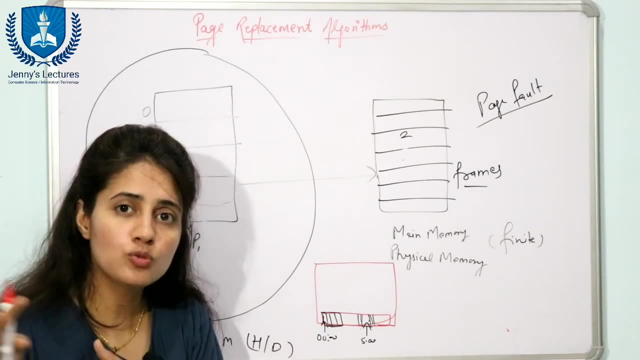 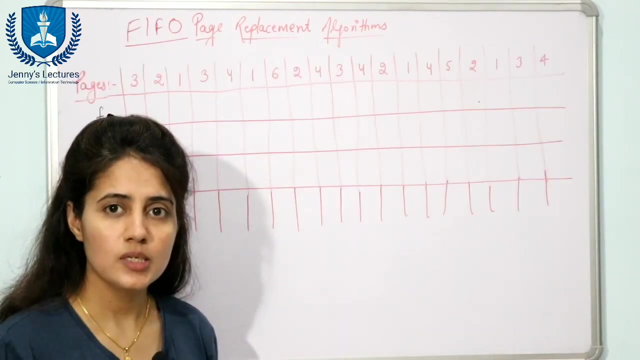 to be choosed. there are many factors on which you will choose which page replacement algorithm is good. one is this: this also: page fault should be less. that algorithm should reduce page fault. that is one criteria. now we will discuss that first in, first out algorithm. now the question is: 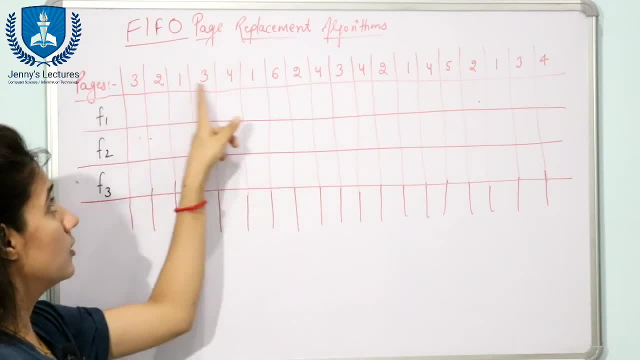 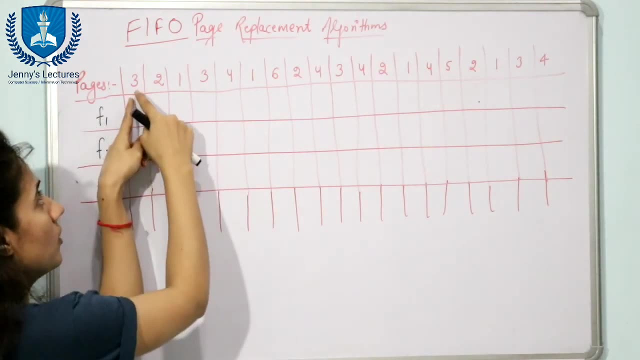 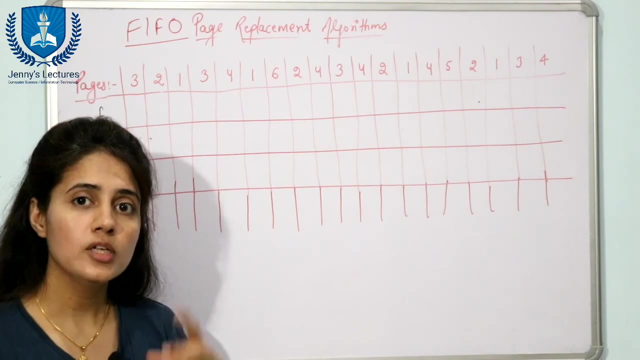 something like this: the reference string is given, that is this one pages reference string for pages. it means CPU, CPU requests pages in this order. it will request first of all three, then page number two, then one, three like this. okay, and you are given only three frames. three frames has been allocated to this process. okay: f1, f2 and. 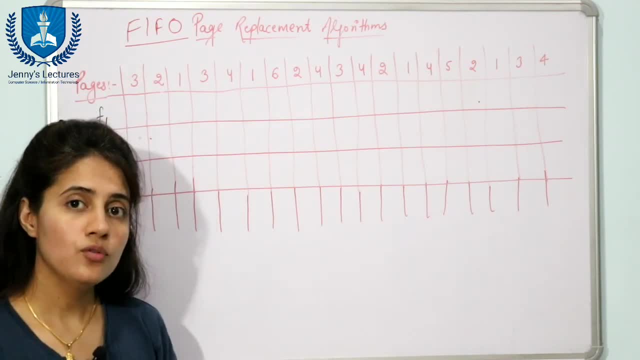 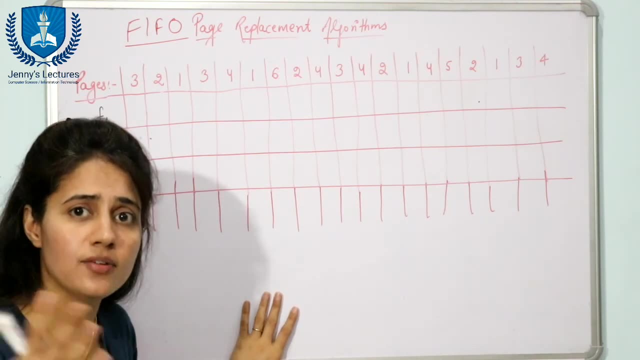 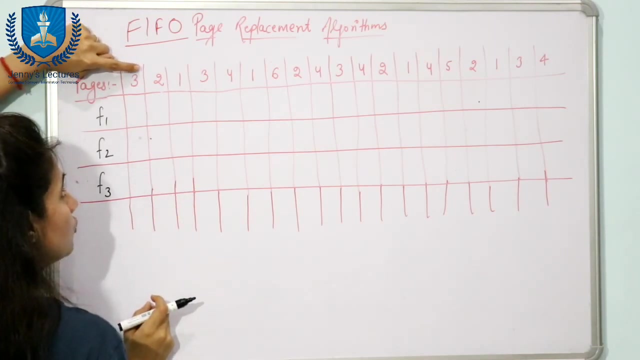 f3. now how you will apply the space replacement algorithm, FIFO, page replacement algorithm: see, and we will also calculate the hit ratio and as well as the page number of page folds. okay, now see the first, first requirement of CPU is what a page number three? okay, now check. frame frame means this is our main. 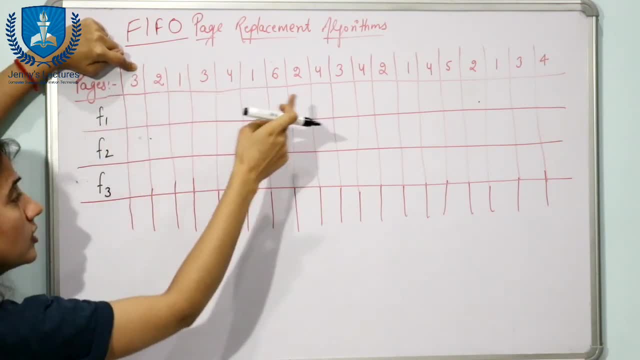 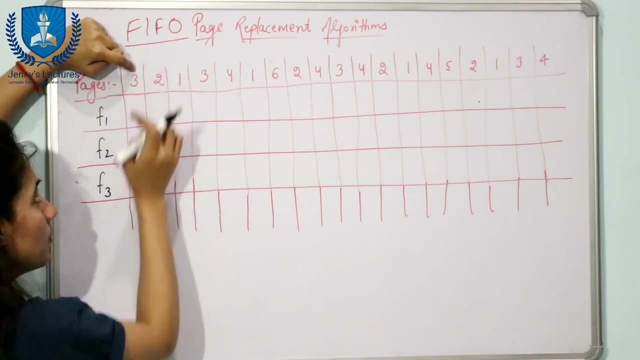 memory. now, three frames are there allocated to this process, allocated to this process. having this, these page numbers, now you check whether you have this page into this main memory. no, this one is empty. this one is empty. this one is empty. we don't have this page number. okay, so we'll swap in this page. 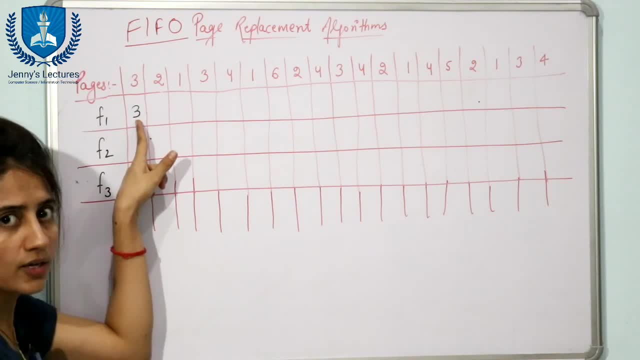 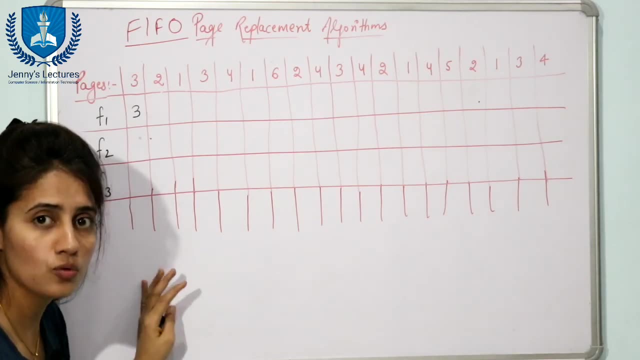 we'll load this page here in frame one, and this is known as page fold, because this page was not available in our main memory. okay, so this is known. you can say a miss or you can say page is not available. page is not available in the main memory, okay. second page now. 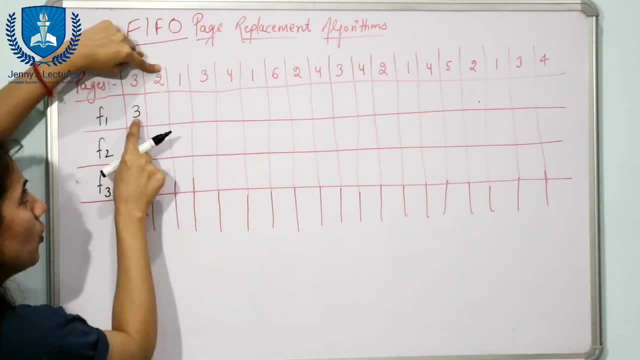 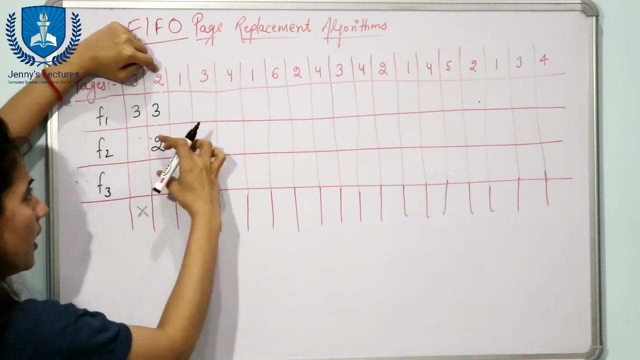 second is page number two. check, we have only one page having number three. we don't have two. so now the operating system will load this page here we have three. in second frame we will put two. see no need to swap out any pagewise. so because we still have two frames left. 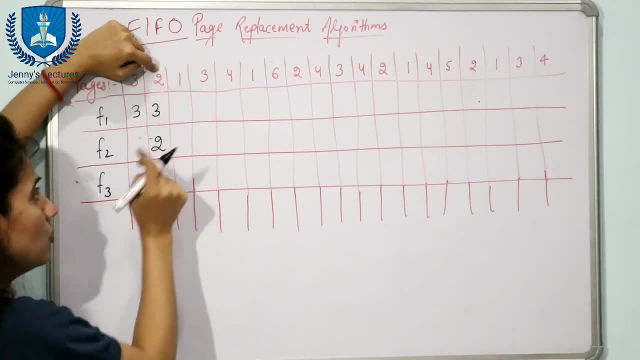 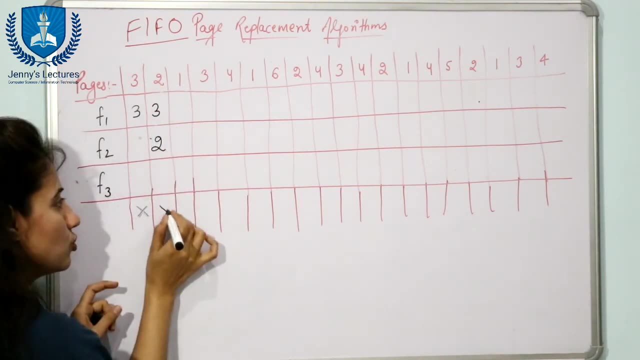 two frames are still empty, so we can put new page into frame two. so this is also known as page four, because two was not available in our main memory. so you can say page was not available or you can say it is a miss. okay, next is one. see we. 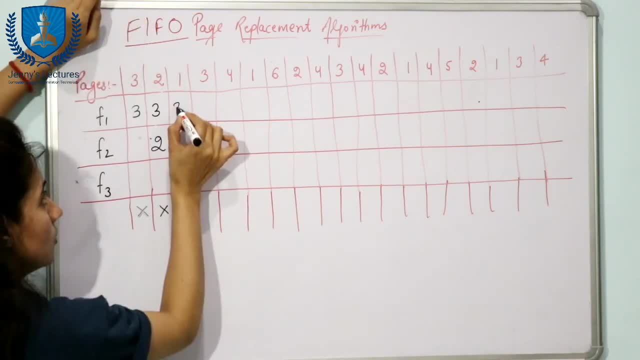 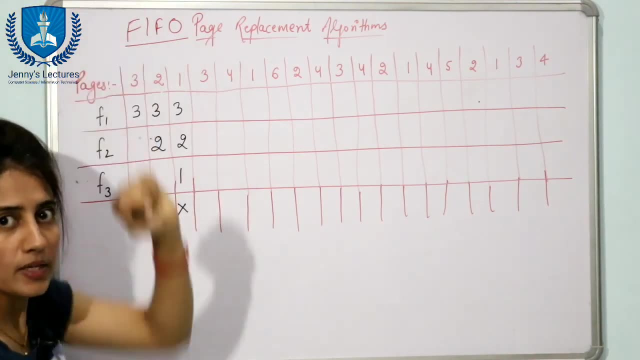 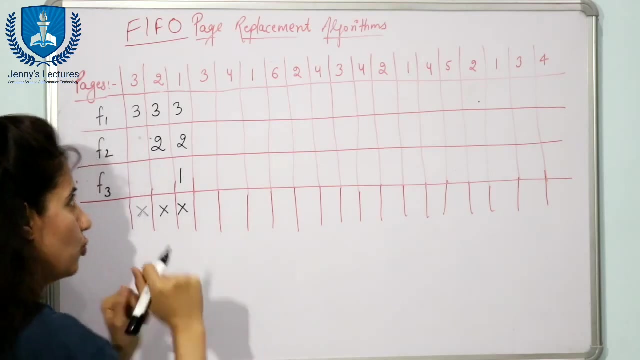 have only page number three and two. one is not available now. three, two. still we have one frame empty, so we will put one here, and this is also a miss, or you can say page fault. now, now, our main memory is full. now. what to do see next page requirement is 3: the operating system. first of all, check. 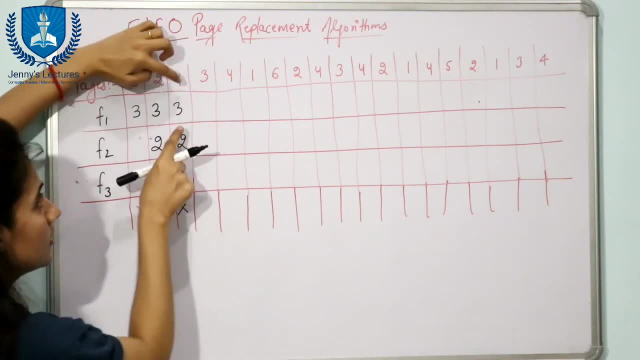 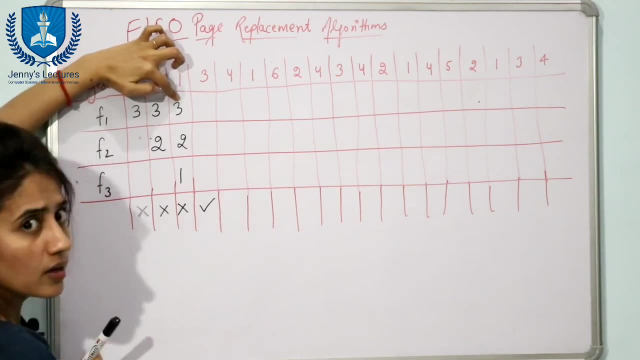 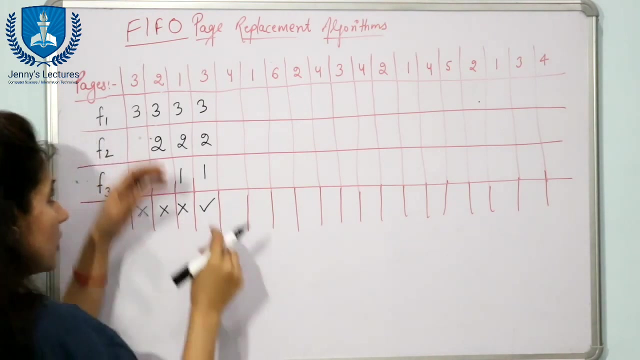 whether. if this page is available in this main memory- yes, this is available, see this one 3. so no, there is no page fault. so page is available. so here, 3, 2 & 1. no need to soap out and soap in. okay, next is page number 4. in this page number available, three to 1. no, this is not available. 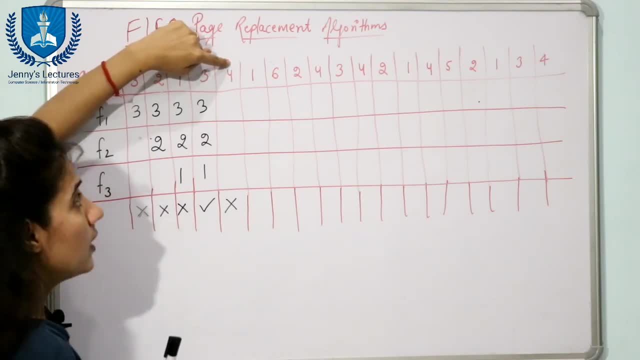 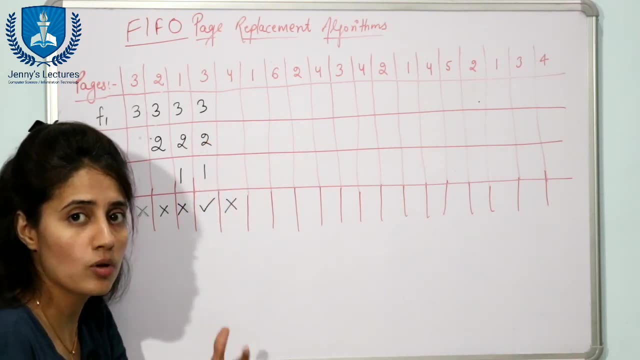 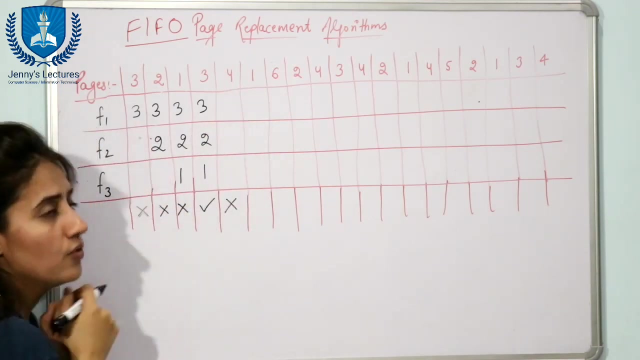 not available. so this is a page fault. you can say a mess. now our memory is full. now you have to swipe out one page. operating system has to swap out one page from main memory to secondary memory. to put this needed pages into the frames, because we have only three frames. 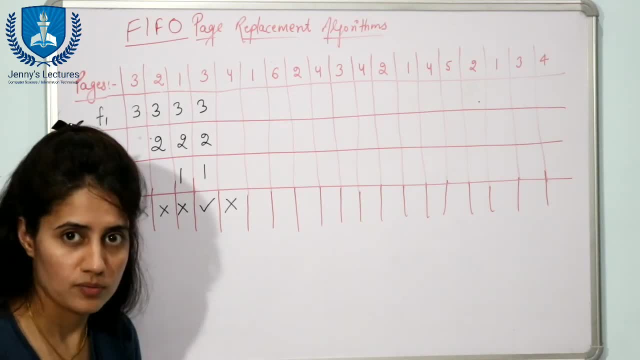 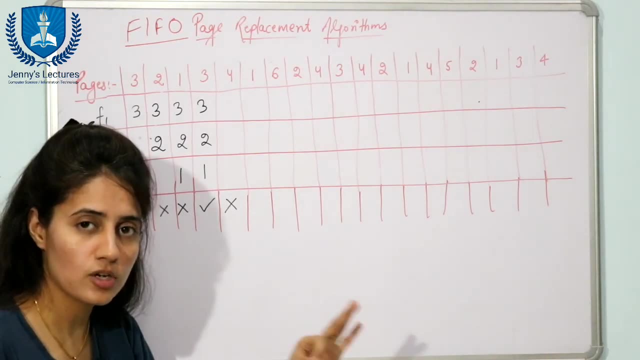 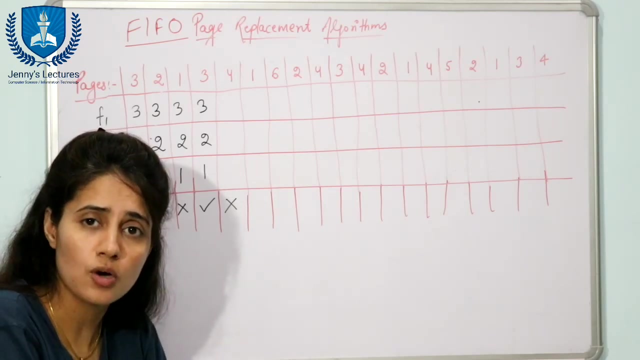 now which page is to be swapped out, which page is to be selected as a victim page in first in, first in first out algorithm. so the page, the oldest page. obviously the names are just first in first out. so the oldest page will be selected as victim, the page which has come first, very first, and for this thing, 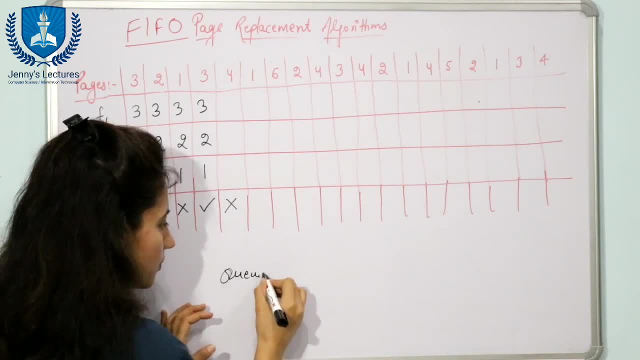 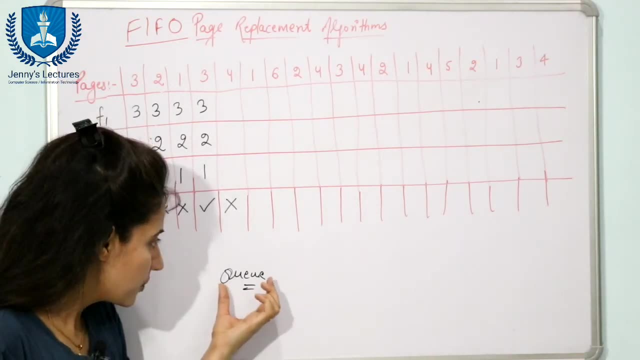 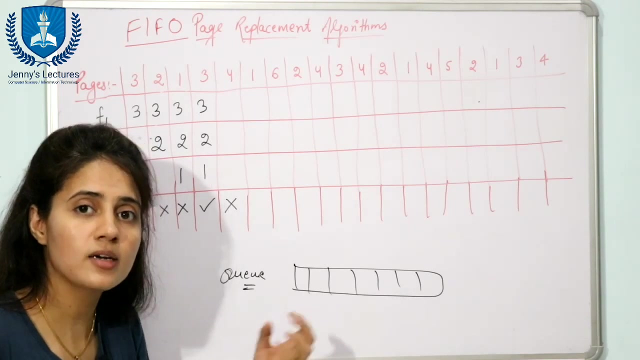 for this thing. operating system will maintain a queue. okay, because the the in Q-Q operates in which manner fit for manner. separating system will will maintain a queue like this and it will put the pages something like this and when, when it has to select a page for swap out, then it will select. 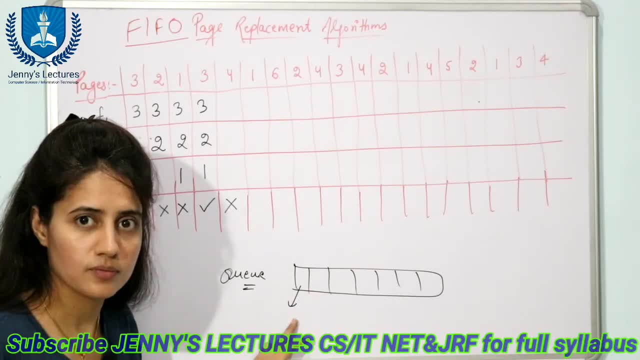 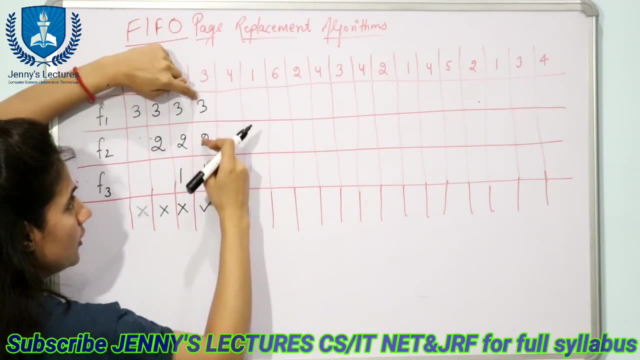 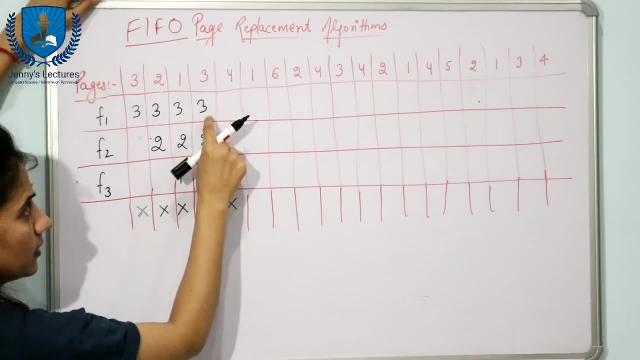 the page from the from front of the page queue. okay, because we we insert data from the rear. now, which page is to be selected out of three, two and one? which pages is the? which page is the oldest page which has come first? this three page? this, this page having number three. so the operating system will swap out this page, so here. 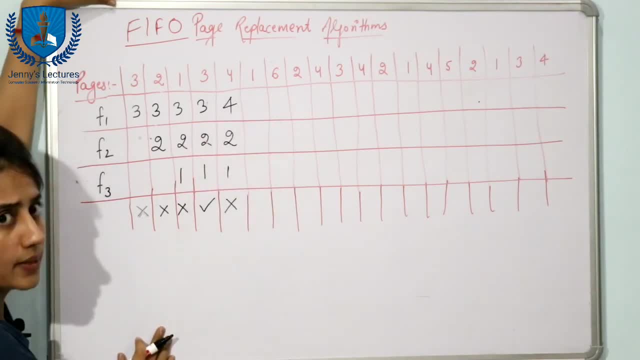 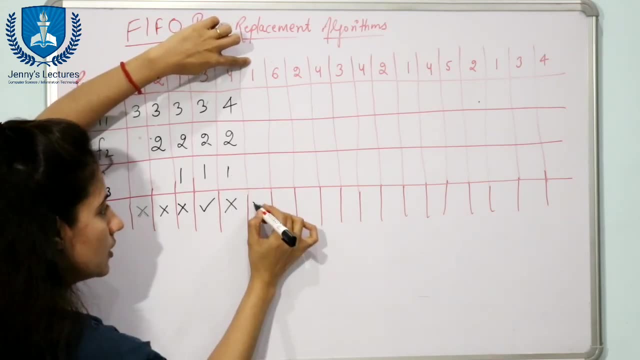 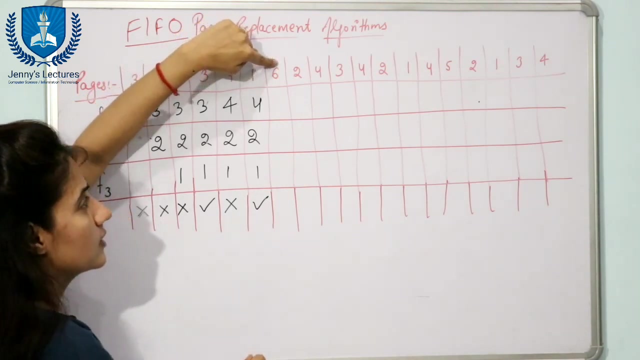 we will put four, two and one will be same. fine, now see for one. this page is already available, so this is a hit. four, two and one page is available, so it is a hit now. next is six. this page is not available now. which page is to be swapped out out of these three pages? which? 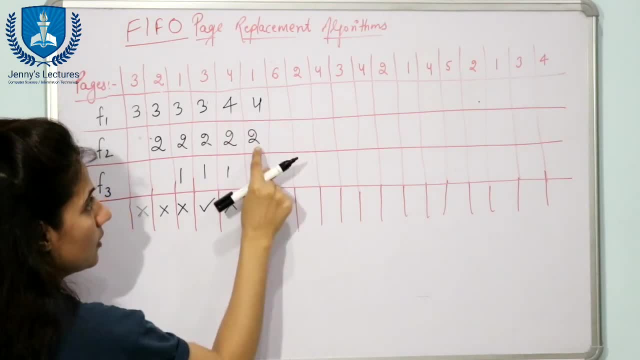 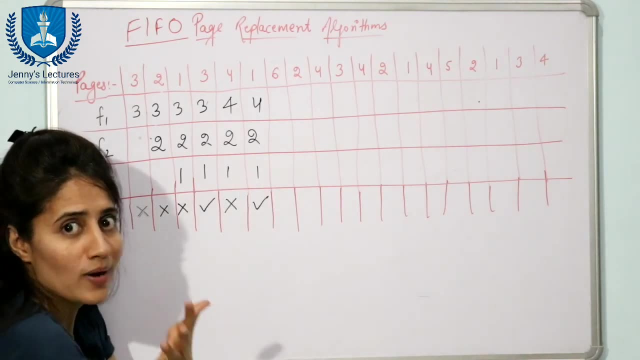 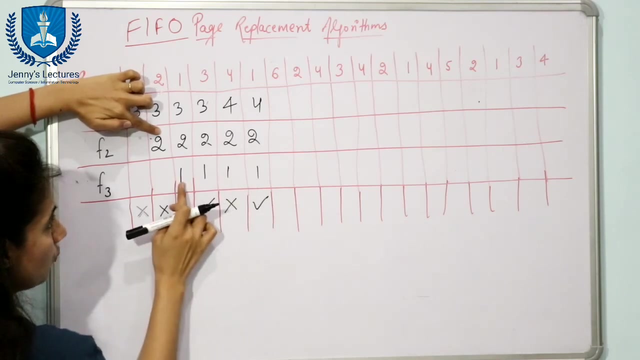 one is the oldest one, see this, four has come here, this two has come at from here and one has come here. so see, the simple trick is. i used to apply this trick. basically, i just see here, only see four is here, starting of two is here and starting of one is here. so 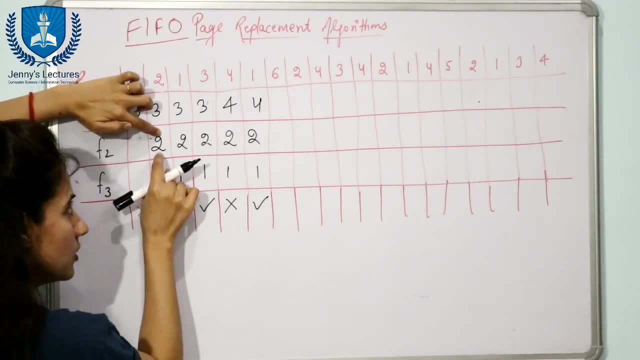 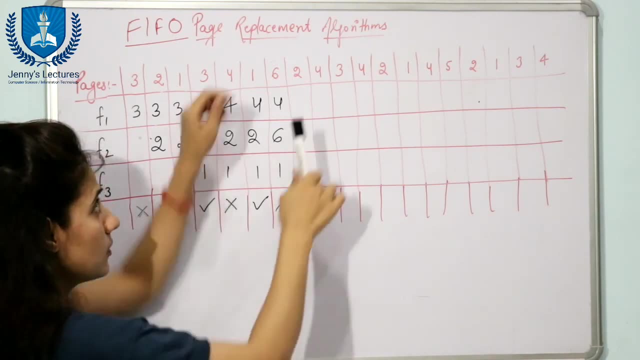 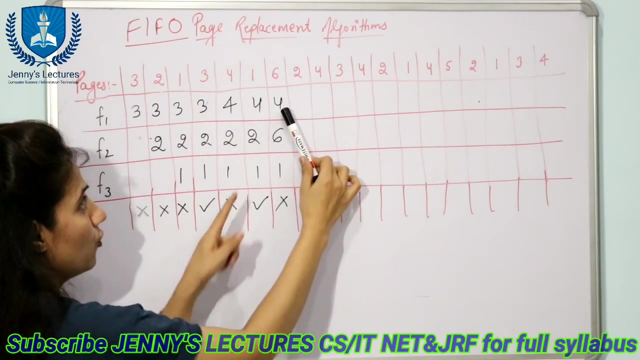 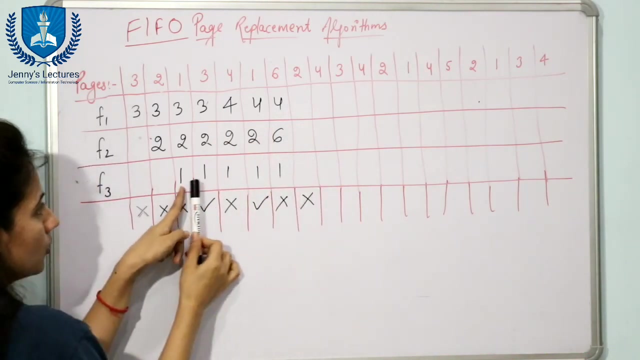 obviously this one is the oldest, so you will choose this page. two, four, six and one, and this is a mess because this, this page, was not available now. two: is this page available? no, so this is a mess. now which page is to be replaced? four has come here. six has come here. only one has come here. only so see after, after looking at. 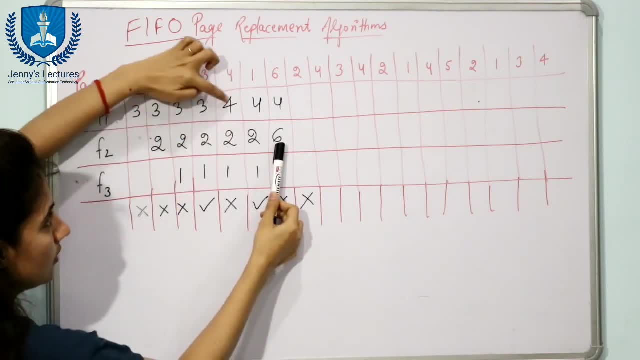 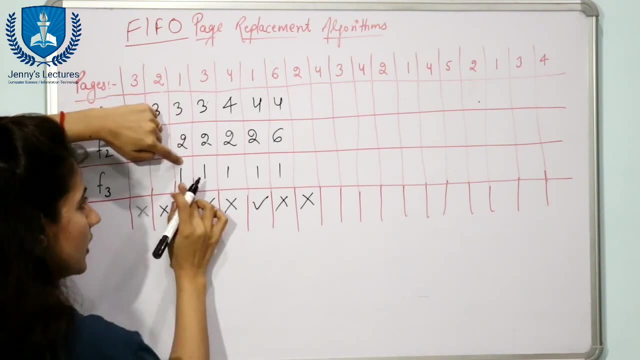 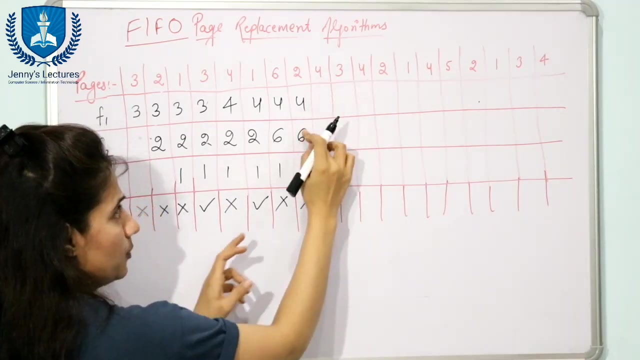 this table after looking at this scenario. six was here, initial point of four is here, initial point of one is here, so obviously this one is the oldest one. okay, so we'll select one, four, six and two. so this is the simple trick i used to apply. next is four. this page is available. four, so this. 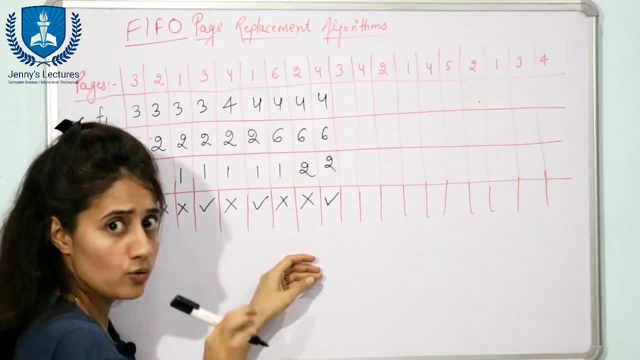 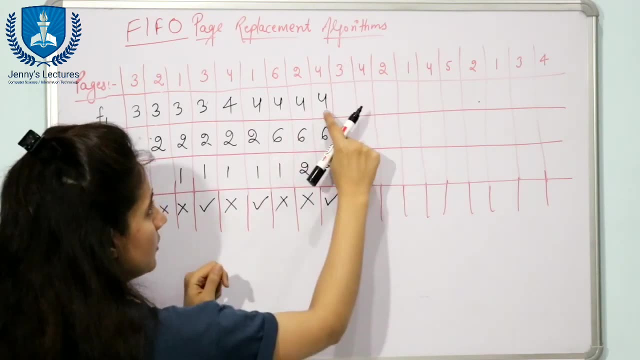 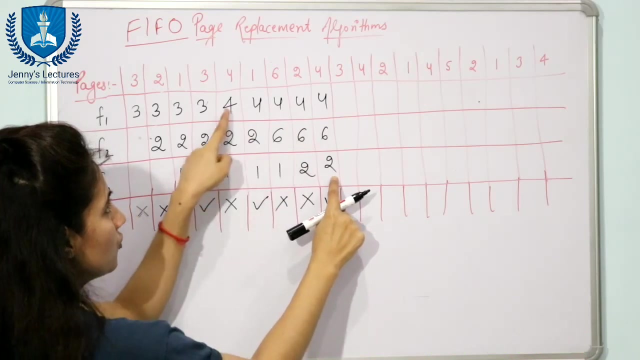 is a hit: four six two. no need to do any swap out swapping now. next is three four six two. this space is not available now. which page is to be selected? see: the initial point of four is here. initial point of six is here. initial point of two is here. so obviously this four is the oldest one, so we will. 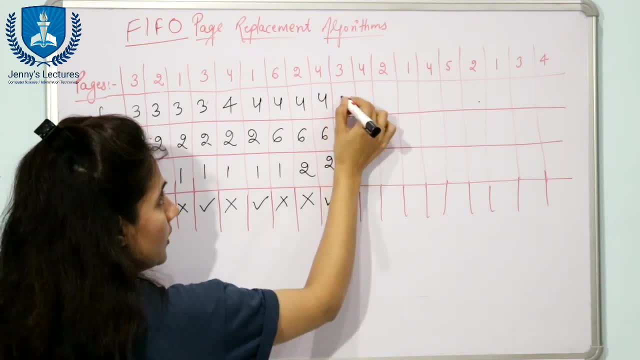 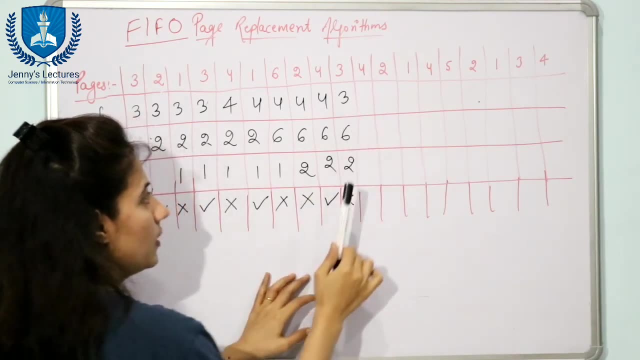 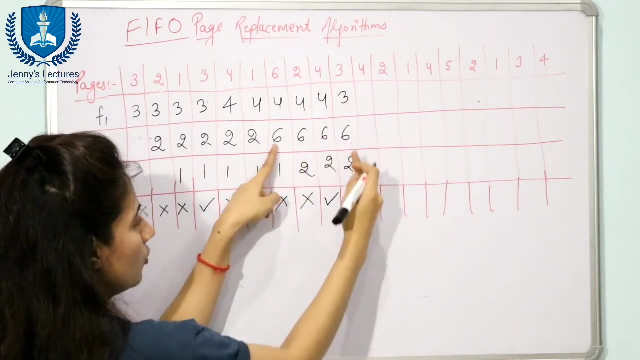 choose this four, so four would will be replaced with three, three, six, two, and here is a miss. now next is four. four is not available. now which page is to be be choosed? initial point of 3 is here only 6. initial point of 6 is here, only initial point. 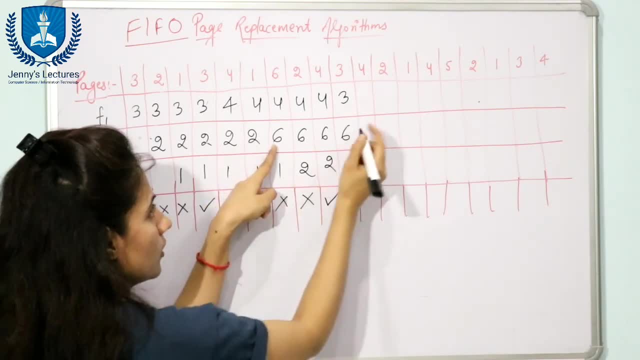 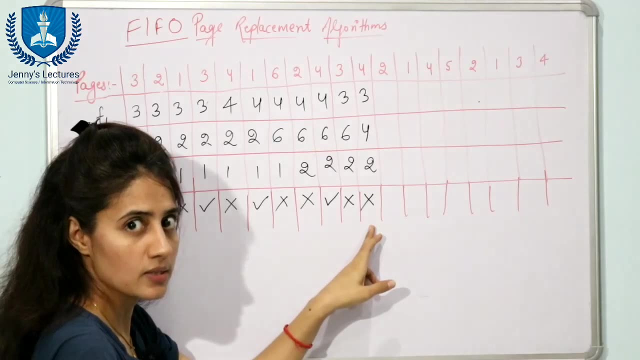 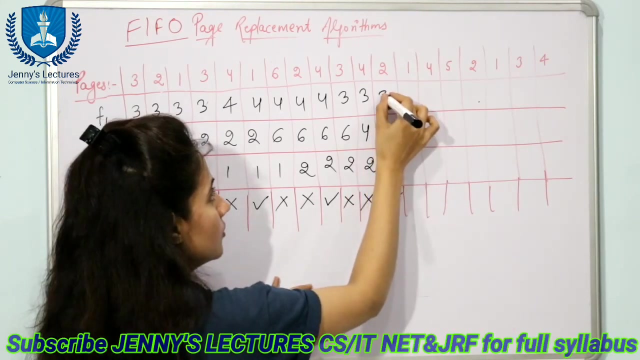 of this, 2 is here only, so 6 is the oldest one, so we will choose 6, 3 and 2. here is also a miss, because this page was not available. next is 2. this page is available, so it is a hit. 3, 4 and 2. 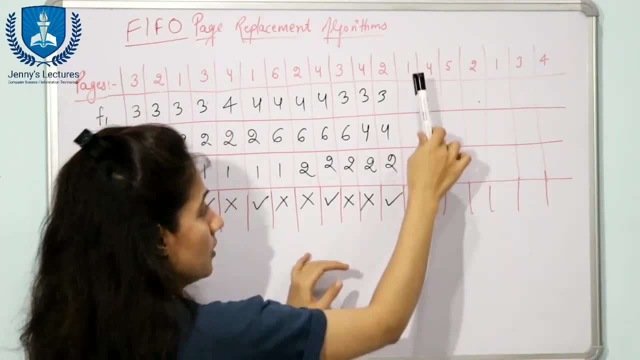 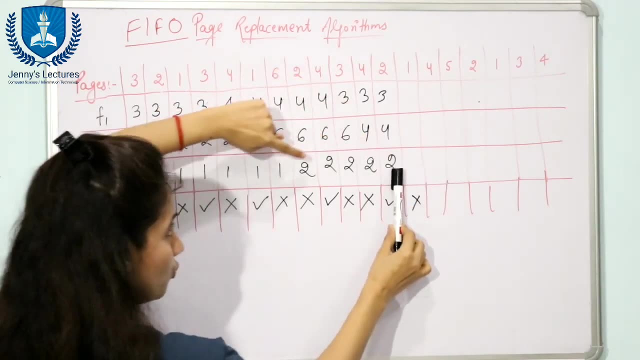 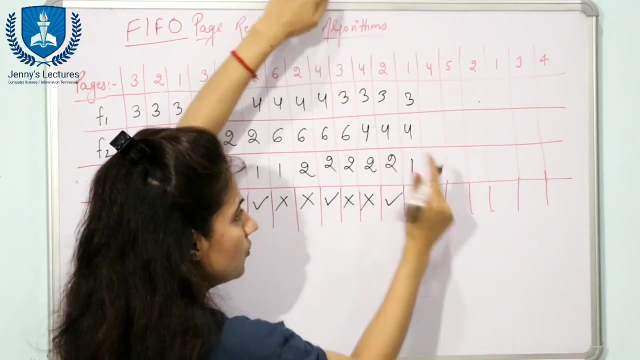 next is 1. this is not available, so this is a miss. which page is to be selected? 3: the initial point of 3 is here. initial point of this one is here. initial point of 2 is here, so this is the oldest one, so we will put 1 here, 4 and 3. next is 4. 4 is available. this is a hit. 3, 4 and 1. next is: 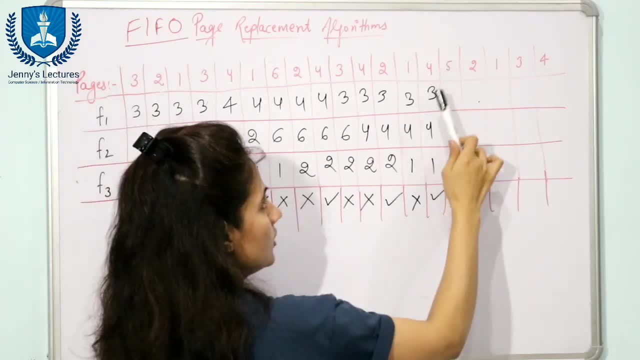 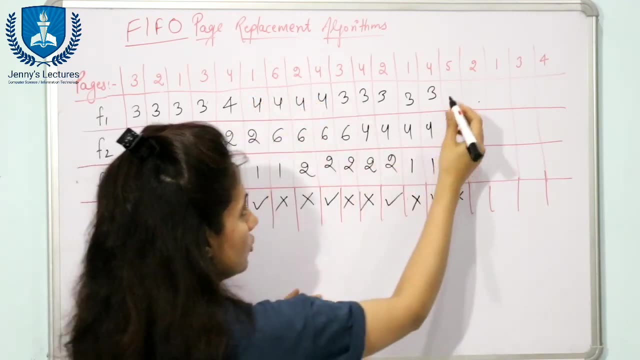 5. this is not available, so this is a miss. which page is to be selected? see. initial point of 3 is here. initial point of 4 is here. initial point of 1 is here. so you select three because this is the oldest one. so here five, four and one. okay, next is two, next two.